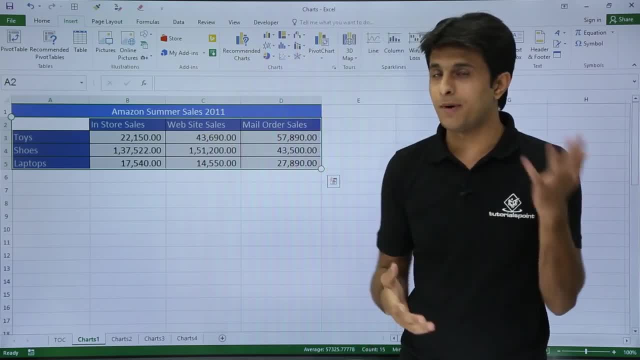 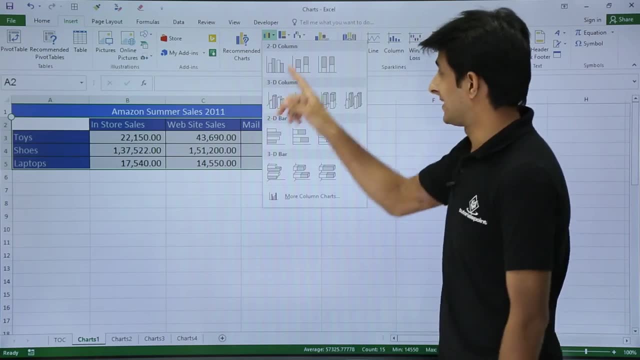 types of charts available: Pi, XY scattered column chart, bar chart. So I'll go with this column chart and I'll select 2D column. 3D column. I have 2D bar. 3D bar, Very simple, basic one. I'll 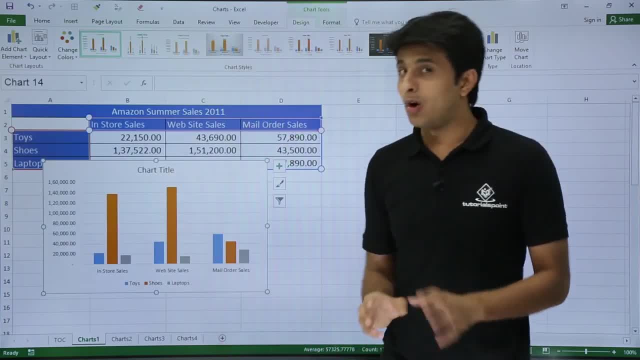 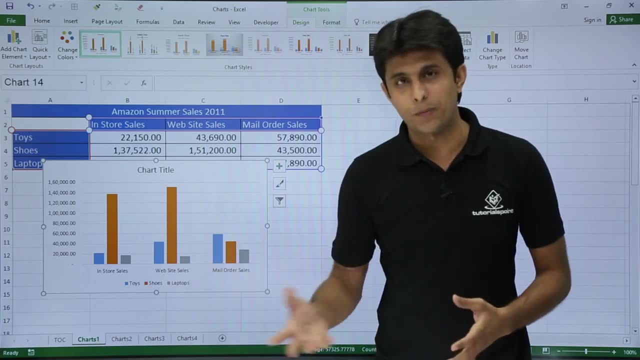 go with the 2D column and that's the same chart which I've got. So Alt F1 key is the shortcut key for your default chart. If your default chart is Pi chart, you'll get the shortcut key Alt F1 for Pi chart itself. Now I'll just try to explain you different elements. 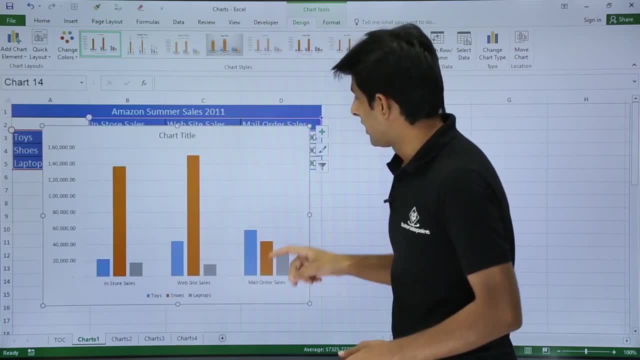 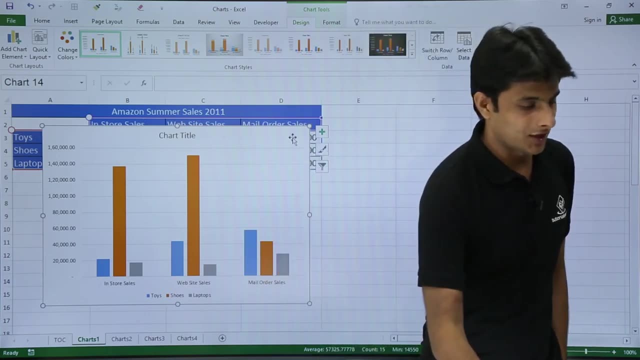 Of a chart. I'm just trying to expand it: Different elements of a chart. Now I'll help you with different elements. How it is, If I keep my cursor at this location, outside it says chart title. I'll just keep cursor outside and now I'll keep my cursor here. It says chart title If I move. 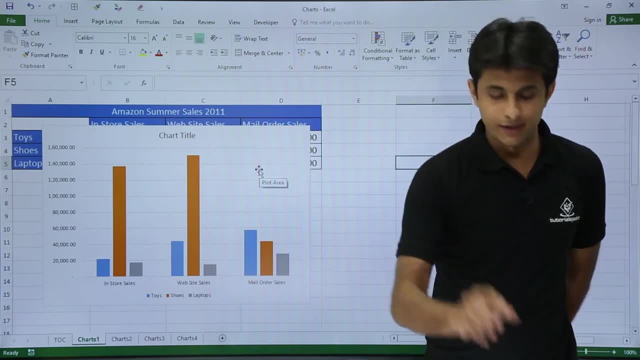 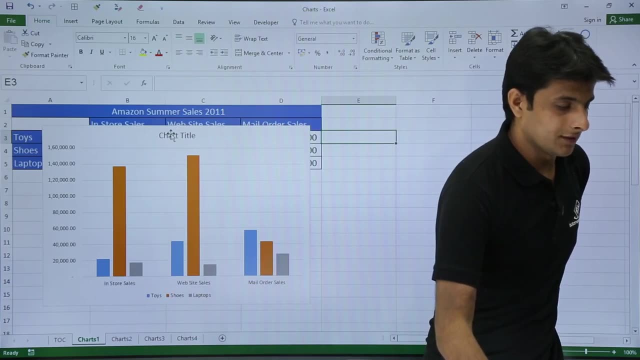 my cursor between this grid lines, it says plot area. Now I'll click on the plot area Now. if you see, this is the plot area which is selected. If I keep my cursor on this place on the chart title, it gives me as the chart title. If I keep my cursor on the left hand side, this it says as: 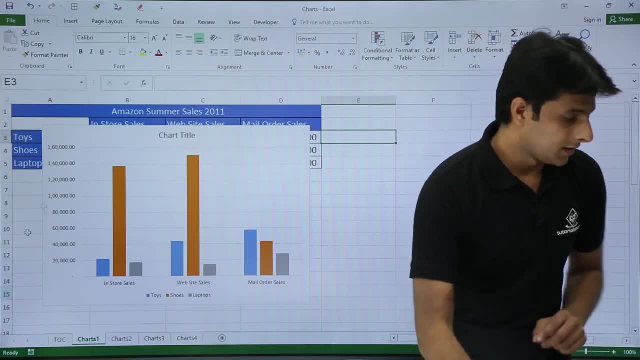 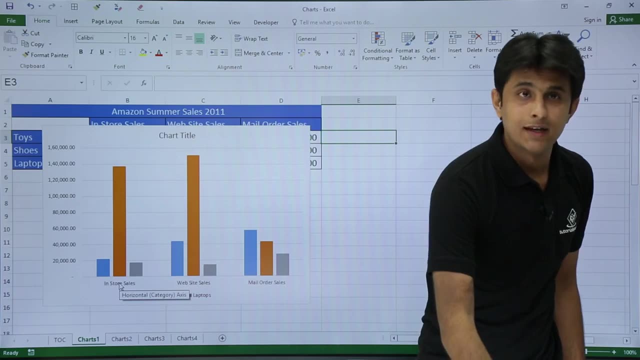 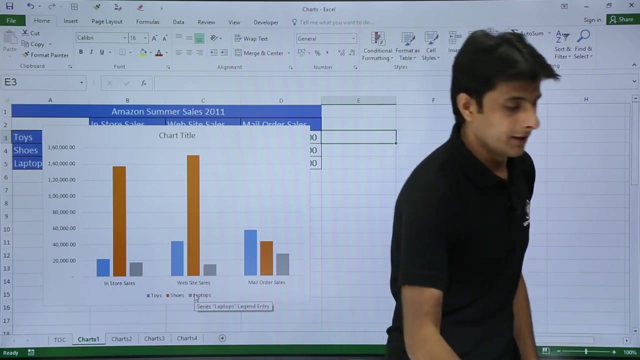 yeah, it says as the vertical axis. Similarly, if I keep my cursor at the bottom, it says as horizontal axis: in-store sales, website sales. Now, if I keep my cursor on this place, it says as series legend. or it says as series laptop legend entry. Similarly, if I keep my cursor 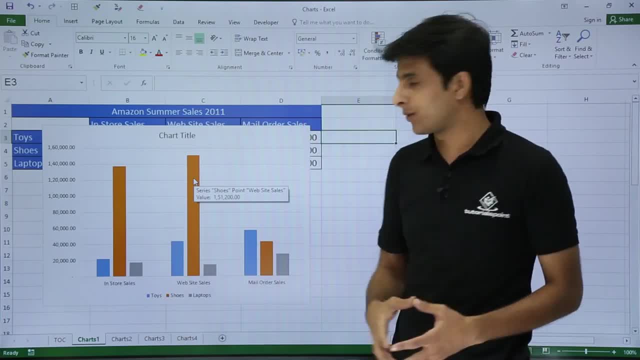 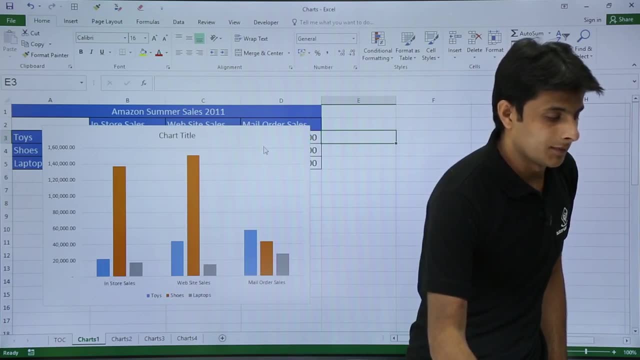 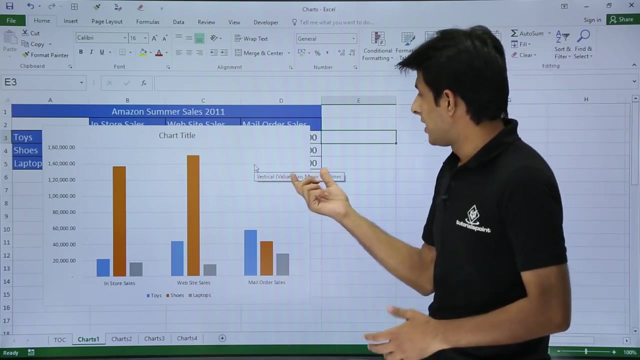 on this, you know columns. it says as series. In short, we call it as a series. Similarly, if I keep my cursor in this line, that's a grid lines over here. So it says as vertical major grid lines. It's difficult to keep, Yeah, So now I've kept the cursor. It says vertical value axis. 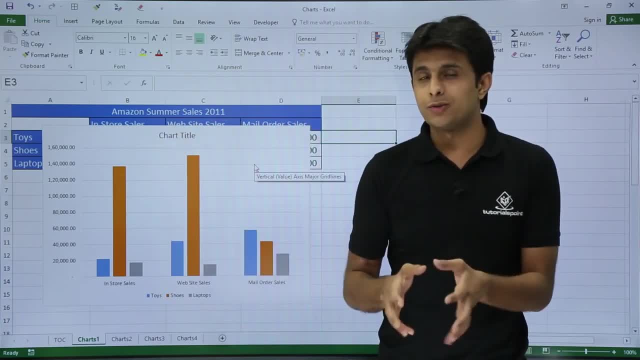 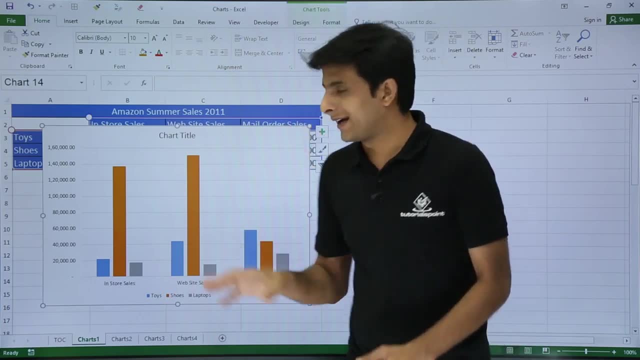 major grid lines. So these are all the elements of the chart. So first thing is, before learning the advanced part, we need to understand what are different elements present. Similarly, when you click on this chart title in the newer version, that is, 2013 and 2016,- it's a very useful option. 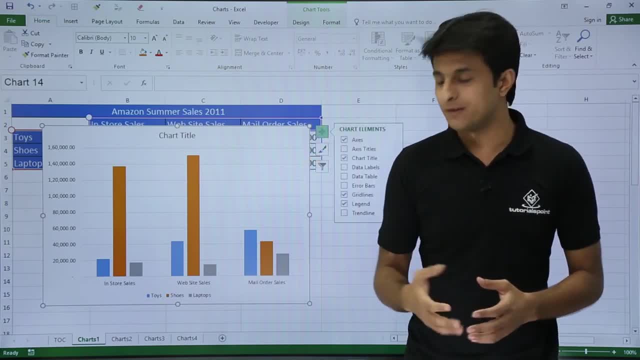 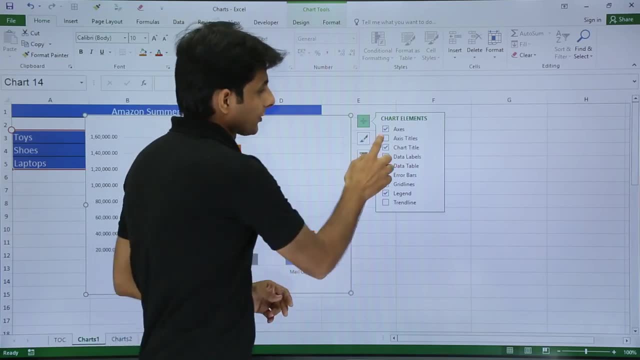 available. So if you click on this chart title, it's a very useful option available. So if you click on the plus sign, it says add and remove the elements. Now, if you observe here what I said was I just click on this plus sign, It says as add and remove the elements. So if you just click on this axis, 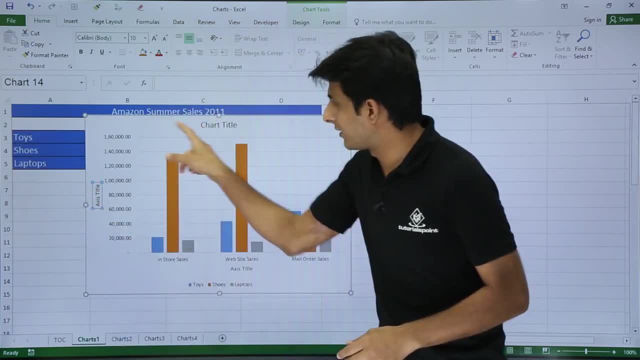 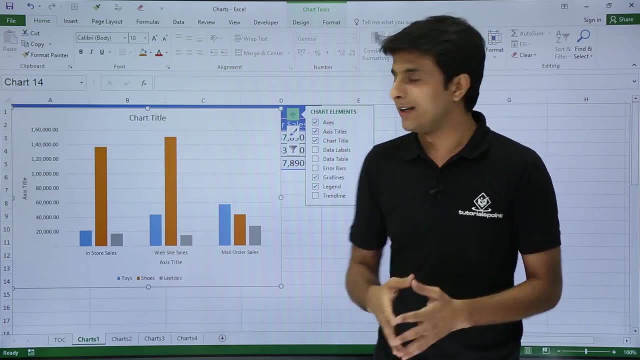 title on the right-hand side and the bottom, if you see there's an access title which is added here. Similarly, if I click on plus, I have loads of options. Just click on the checkbox. You will add. remove checkbox, It will delete. Next is there is the option for style and the color, which is 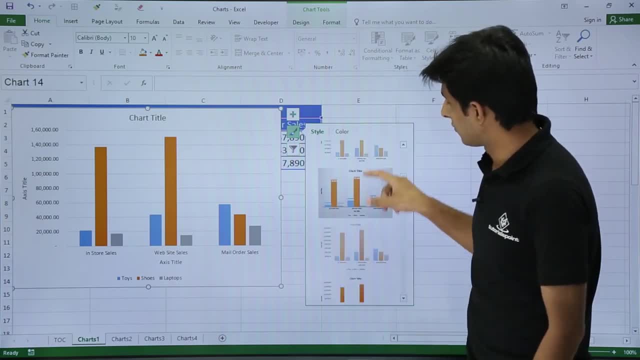 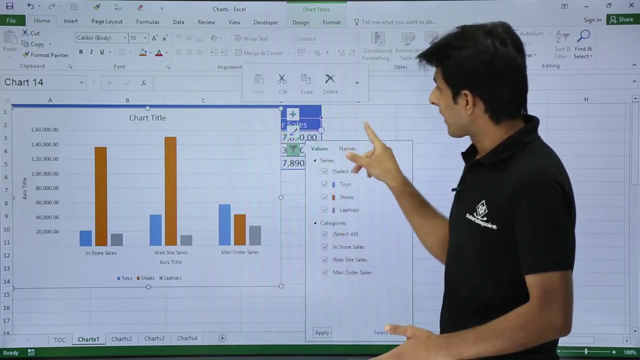 available inbuilt by Microsoft Excel. You can choose the size you know, different formats available here. Similarly, you can filter out the options which you'll be seeing in detail. all these three options. Next is, if I keep my cursor in this place, inside this chart, type, article, chart area, my data. 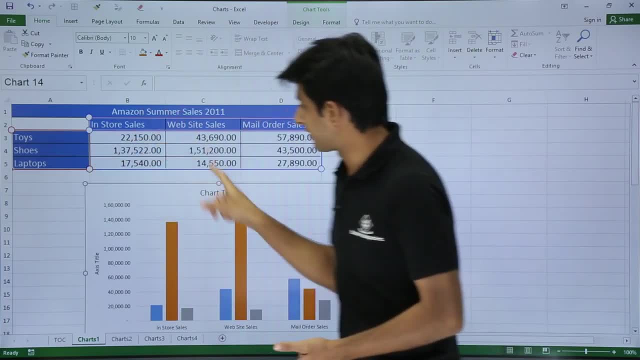 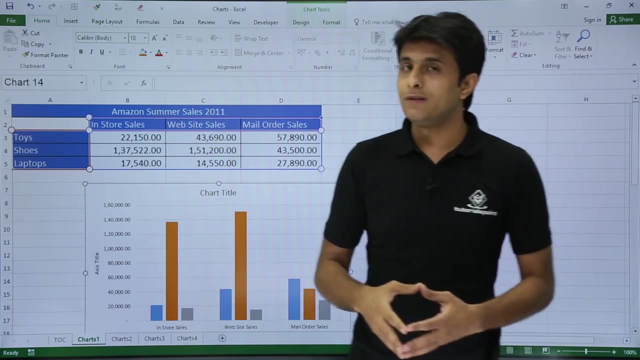 at the back end will be highlighted. If you see, my data at the back end is highlighted by some colors. If I keep my cursor outside, it goes away. If you keep your cursor on the chart area, you see it is highlighted. Now one more thing is: if you keep your cursor on your chart, there are some 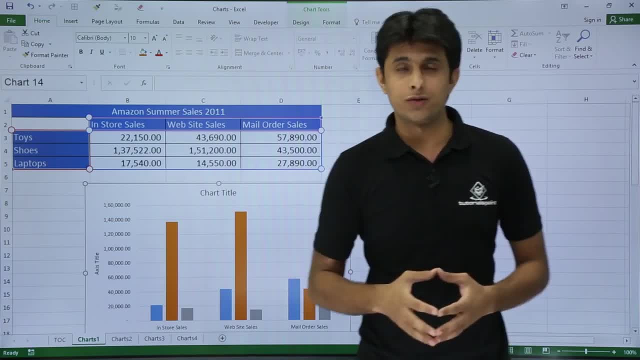 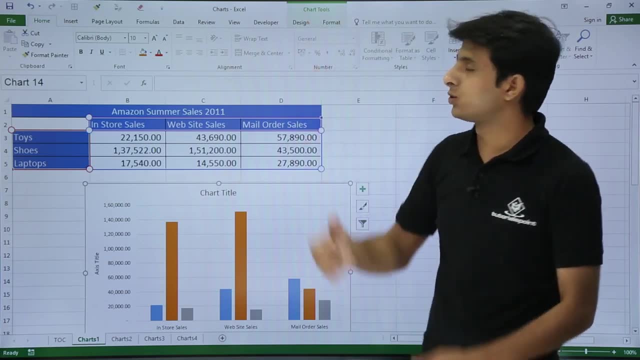 tabs which will be appearing Now depends on which version of Excel you're using it. the names keep on changing. Now I'm using Excel version 2016.. If I keep my cursor on the chart area, I get chart tools. 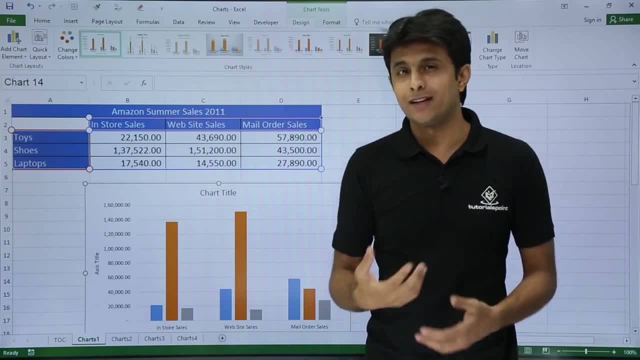 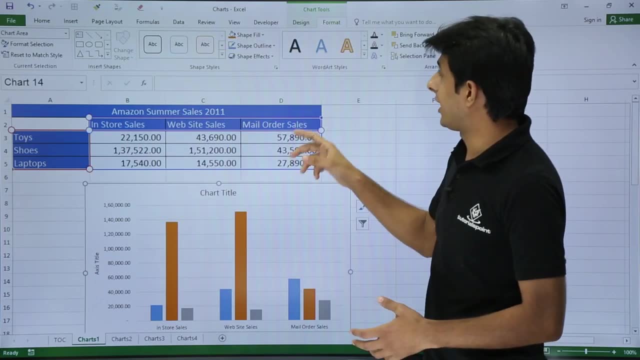 One is for design and format. Designing is for, again, adding and removing the elements, changing the format, and I mean changing the chart types, Whereas the format type will help you to change the colors, add some images, shapes and also you can see us moving backward and forward different. 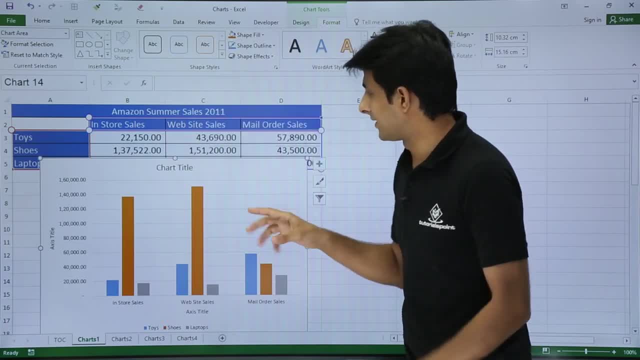 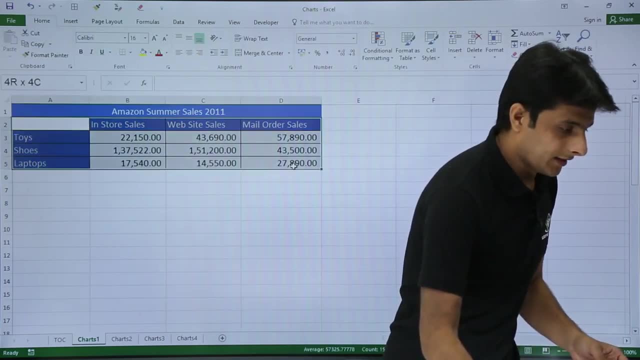 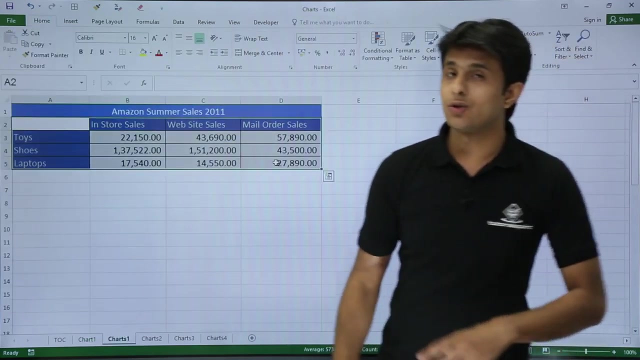 options available. So this is the shortcut key by which you can get the chart in the same sheet. The shortcut key was alt F1.. Now I'll delete the chart. Now I'll delete the chart here, and yeah. Now the next one is another shortcut by which you can get a. 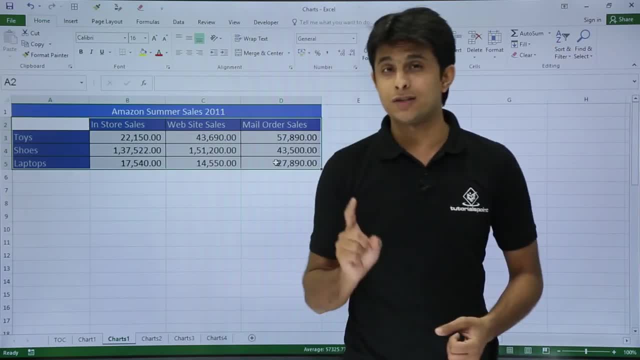 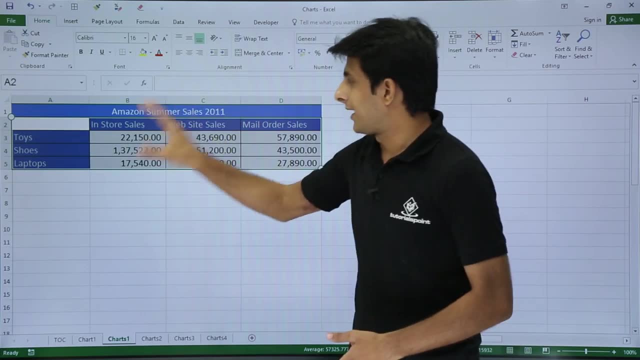 chart in some other sheet just by using a shortcut key in just one second. How do you get it? First option is: first thing is you need to select the data without the you know the column heading itself and have that. that's the title, and you have to press shortcut key from a keyboard that. 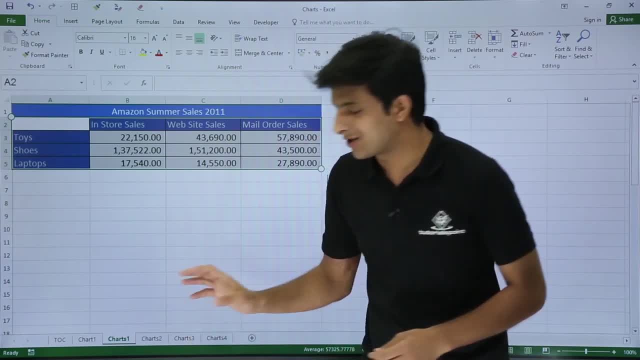 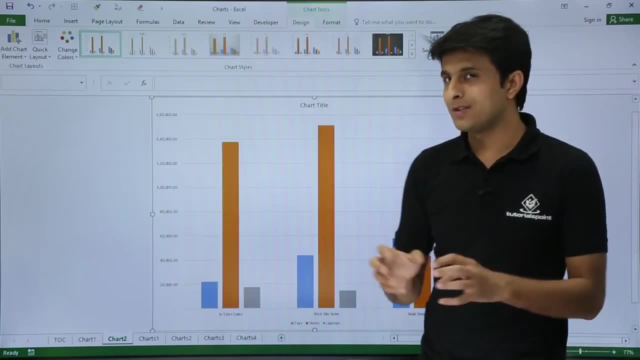 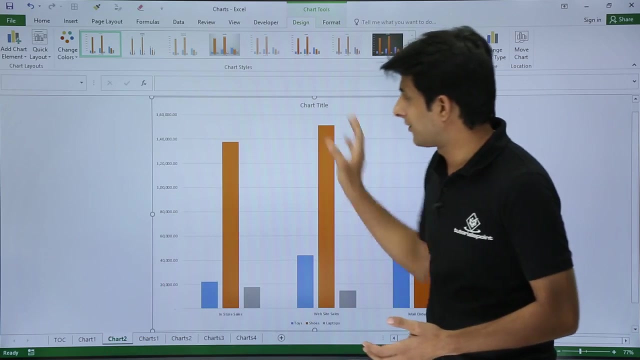 is F11 and if you press F11, you'll get a separate chart sheet. I'll press F11.. F11.. So once you press F11, the same chart which earlier was inside the sheet. now it has taken a parallel, separate space- You'll see there's a chart 2 sheet where you have the data here and the same.